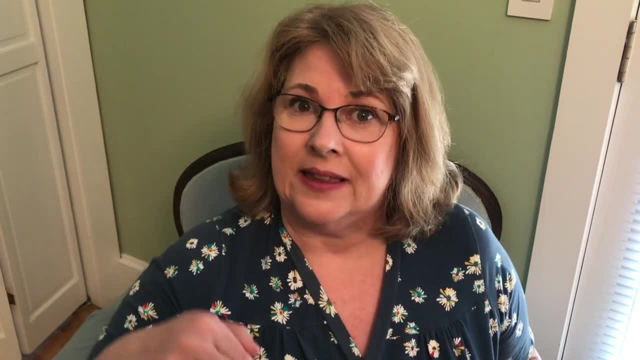 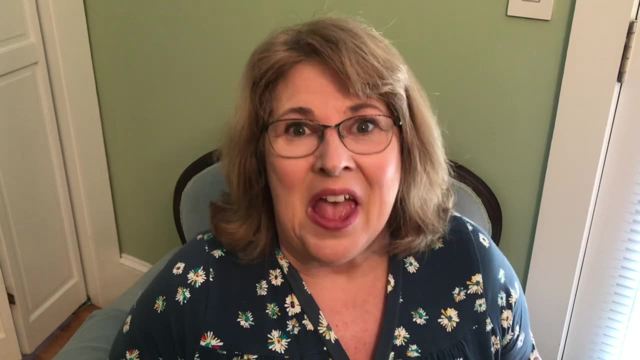 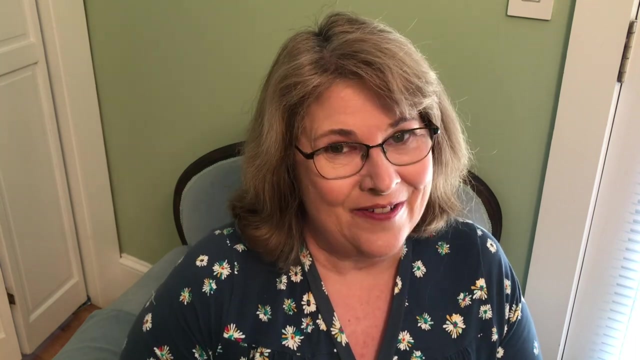 can participate. Everything I talk about will be linked down in the description box below and if you have any questions, hit me up in the comments section. So the first is that you are to use fabric from your stash, so don't go out and buy any new fabric, Use a free pattern. that 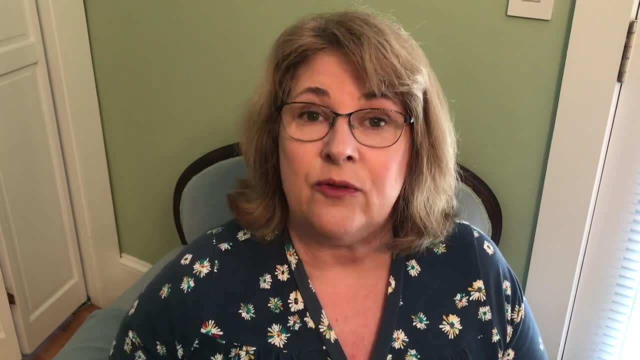 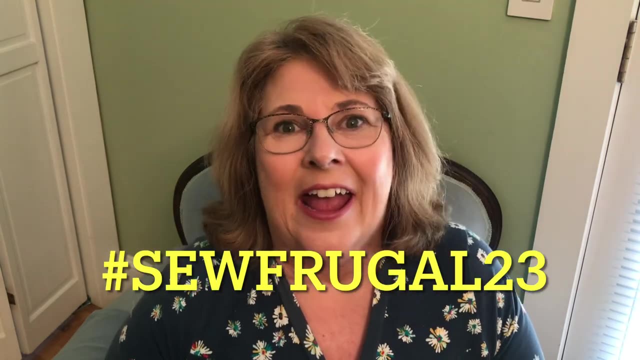 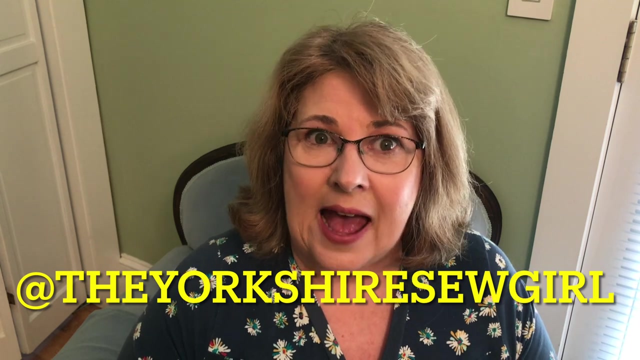 is free to anybody to sew a garment for a person in the month of March and then post that said garment to Instagram and use the hashtag Sew Frugal 23 and you will need to tag at the Yorkshire Sew Girl and at Frugalissima in your post. 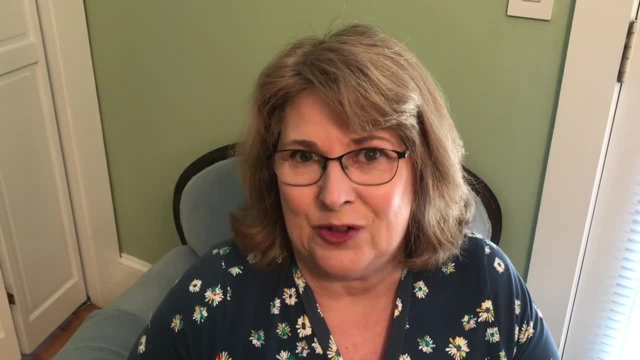 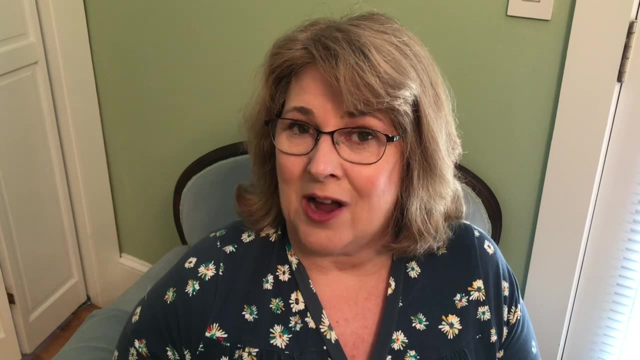 So that they can count and include you in the prize drawing- and there will be a lot of prizes. So if you have any questions, hit up below in the comments section and I'm going to move on. But first I want to tell you about what I'm wearing. 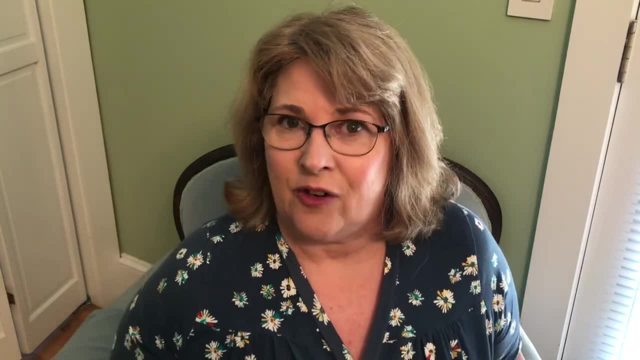 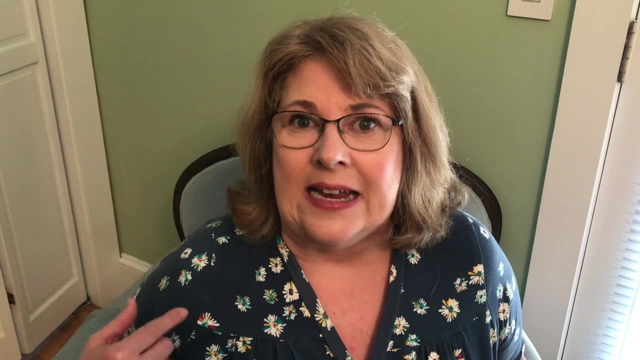 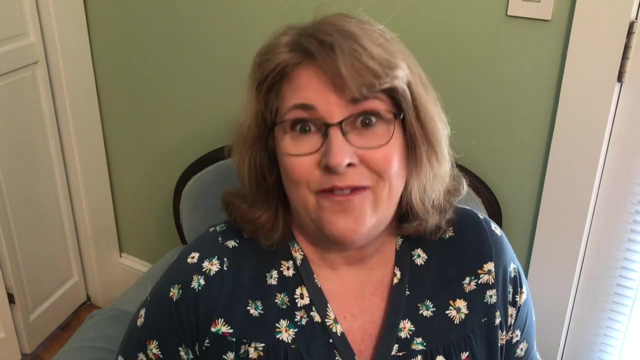 Today I am wearing the Westcliff Dress by the Friday Pattern Company. I sewed this about two years ago in this cotton jersey from Art Gallery. It is the Hazy Daisy Marine Print and I do know this is still available. Though my favorite person to sew for is me, I do sew for the little. 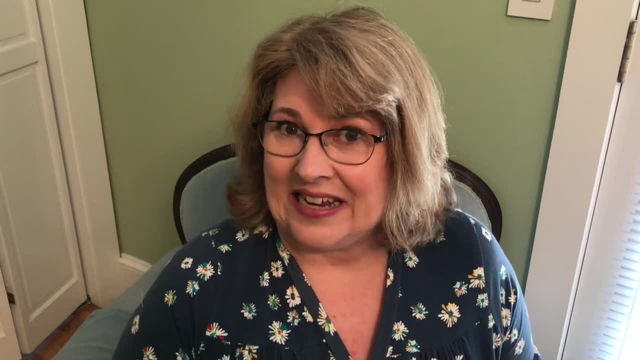 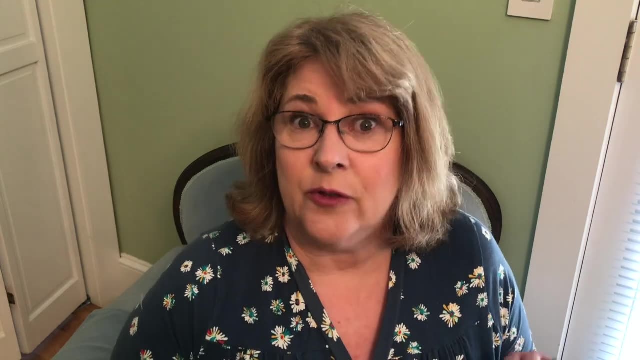 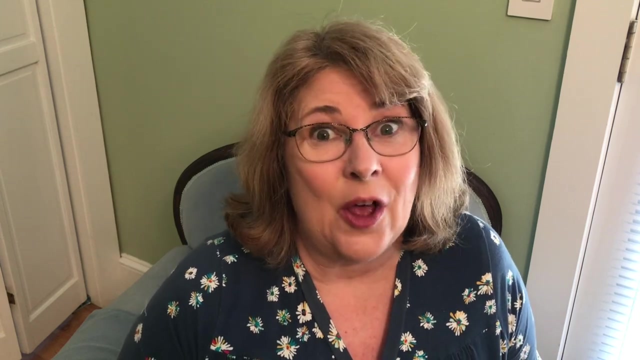 people in my life a good bit, And I thought today I would focus on nine children's patterns that you will want to sew. I have sewn several of these patterns already, Some are new to me and there are some definite sews on my list, So let's jump into the patterns I've selected. The first two that I've selected are both leggings patterns, So mainly for girls, but boys do like leggings too, when they're little, And I have a couple of patterns that you can choose from. One is the Petite Pegs from Patterns for Pirates. This goes from a size preemie to 12 month. 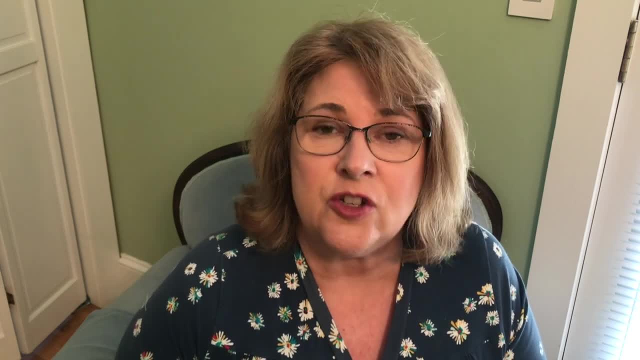 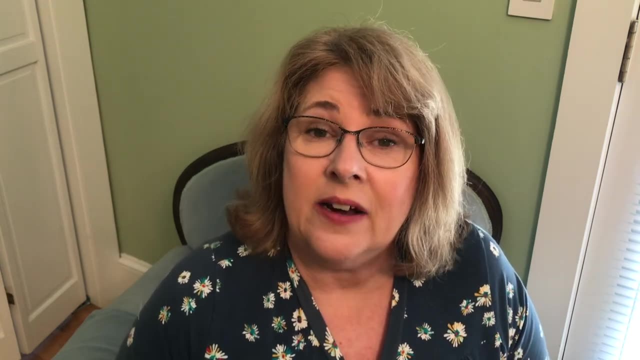 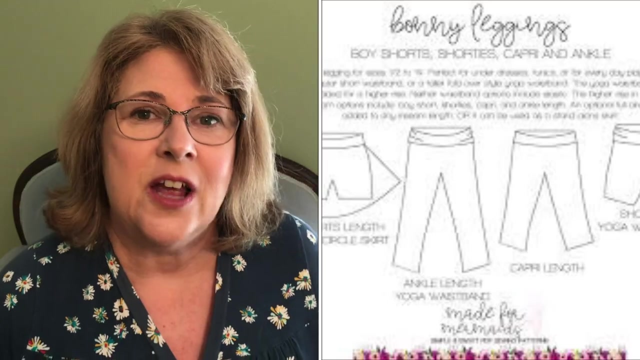 And Pattern for Pirates has several free patterns you may want to check out on their website. The other leggings pattern I want to talk about is the Bonnie Leggings from Made for Mermaids And this goes into a higher size range. I'm going to be linking the patterns, So links to where you 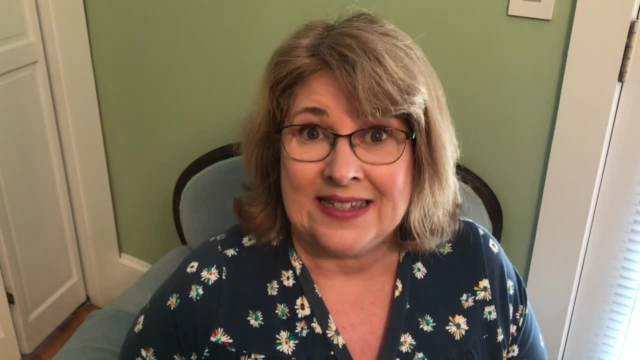 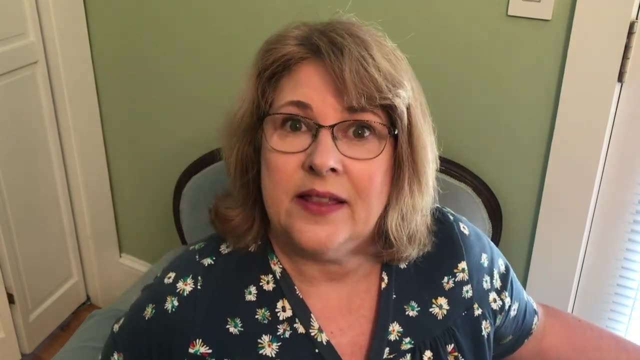 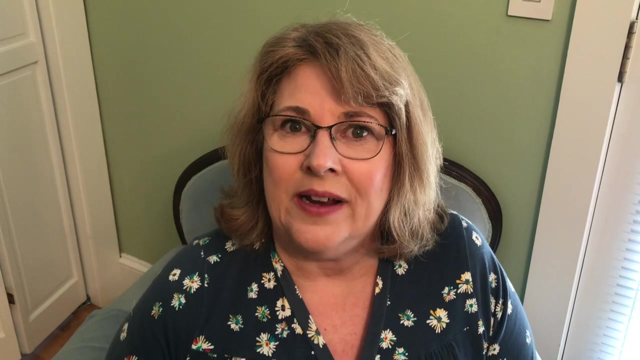 can go get the free patterns and information about the sizing in the description box below. I've made both of these and I have definite plans to make the Bonnie Leggings for Baby Girl. I've made her appear just a couple months ago in a zebra print fabric. I'll insert a photo if I can. 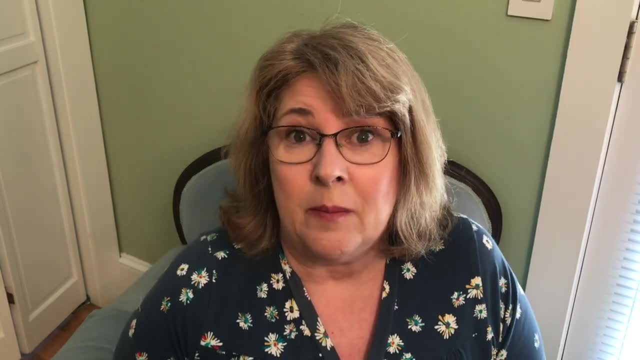 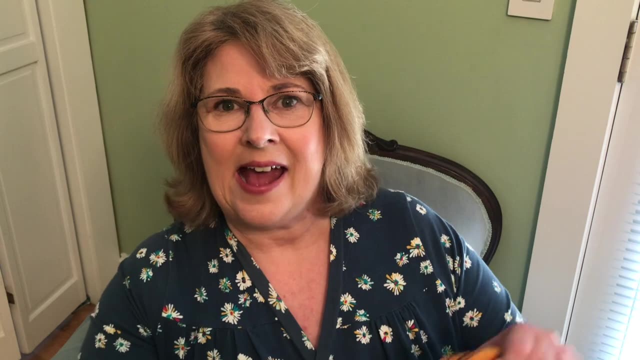 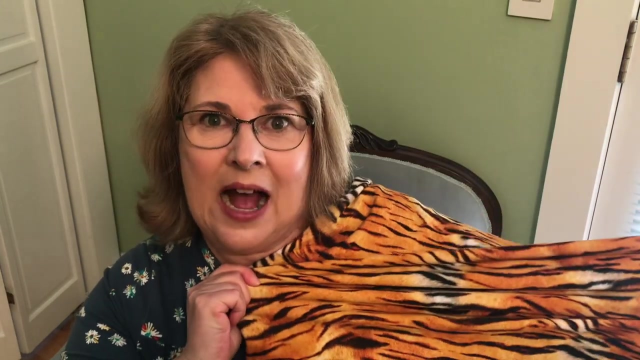 find one of her wearing them. She's been wearing them on constant repeat and wants them as soon as they come out of the wash. So I have this in my stash. It's a Robert Kaufman cotton lycra. I have some tiger and I have some. 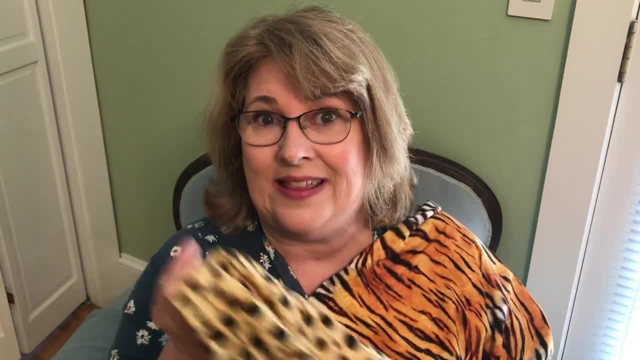 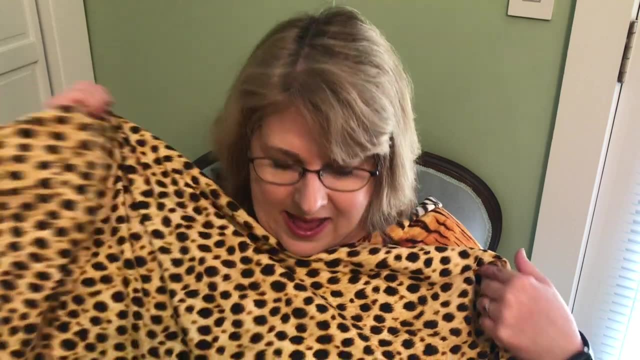 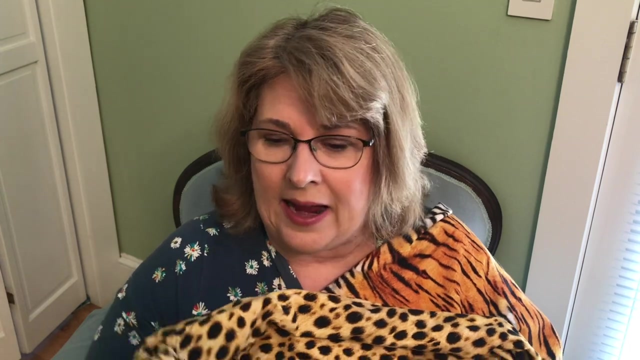 cheetah And I think she would enjoy this as well. She's really into animals right now and I think this would be fun. I have a yard of each left. I've got a new baby niece who's going to be due in April, So I may be sewing some up for her as well. I would like to sew. 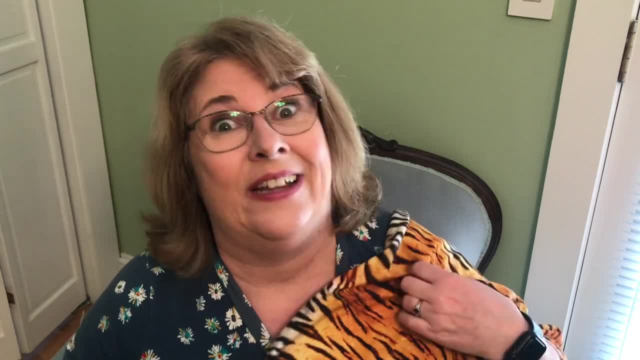 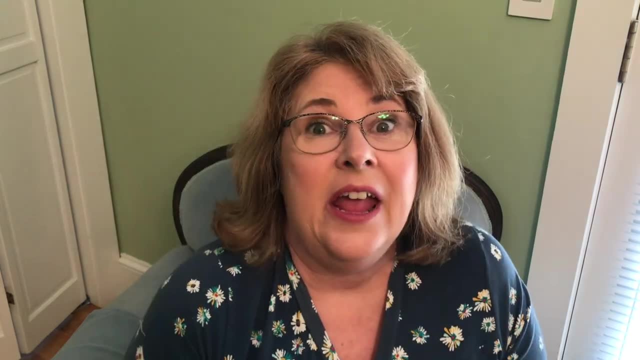 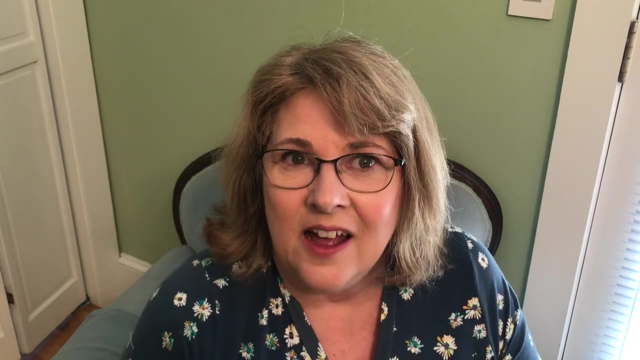 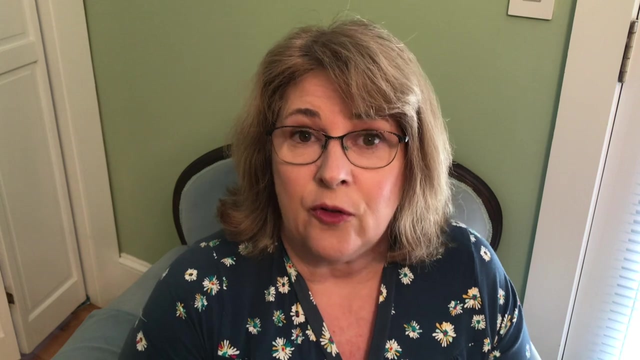 all of this up this month and get it out of my stash. I think I have a few things in mind for this month. If you've followed me for any length of time then you know I love the aesthetic of the Modern Vintage of Violet Field Threads patterns. They have several free patterns and I'm going to talk. 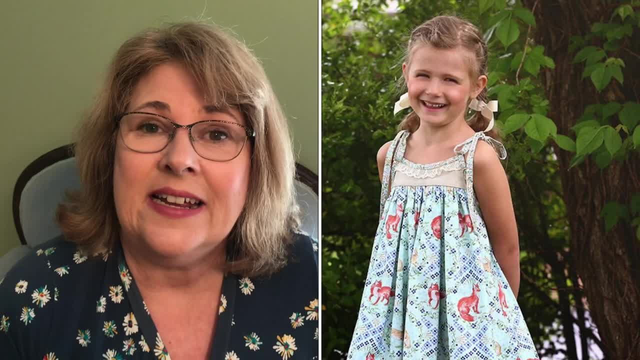 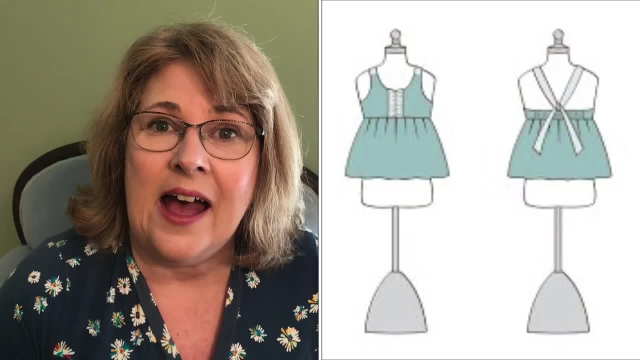 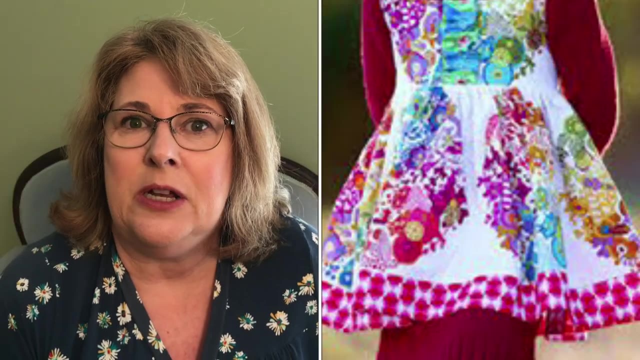 about two of them today. The first is the London Dress, which is a very sweet sundress with a ruffled hem- hem, and the other is the lola top. this top is really versatile. i think that it would be great in the summer with a linen weight, but you could use it as a pinafore if you sew it up in a little. 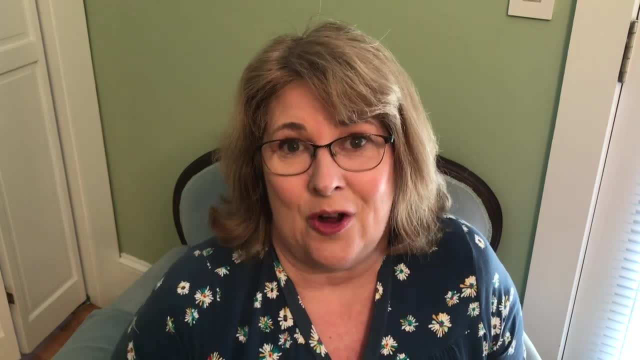 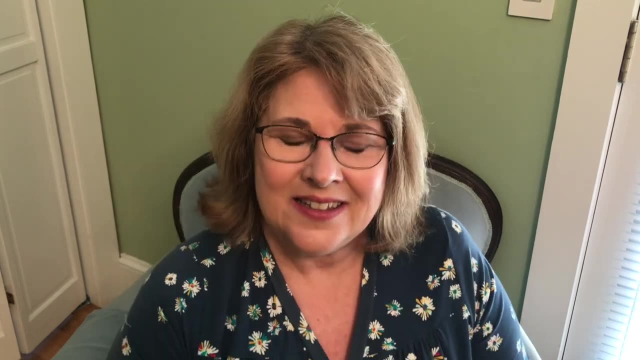 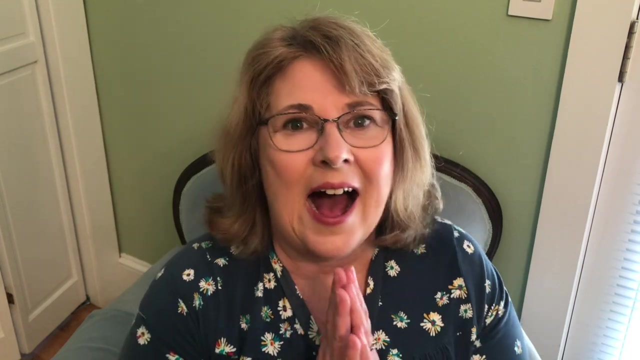 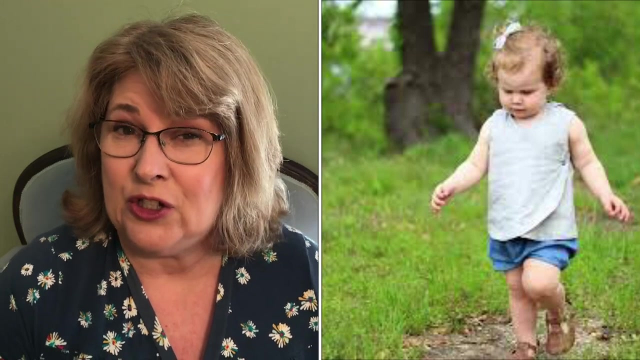 heavier weight fabric. so, so cute. i love the aesthetic of the modern vintage. next on my list- and it's got a little bit of the vintage vibe- is again a couple of baby girl patterns. i am definitely going to be making the petal wrap from twig and tail. i will make it in a size. 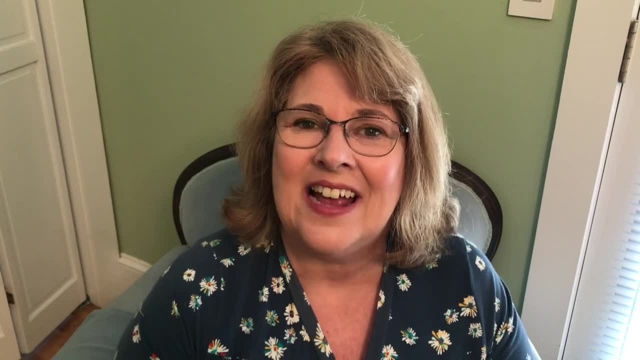 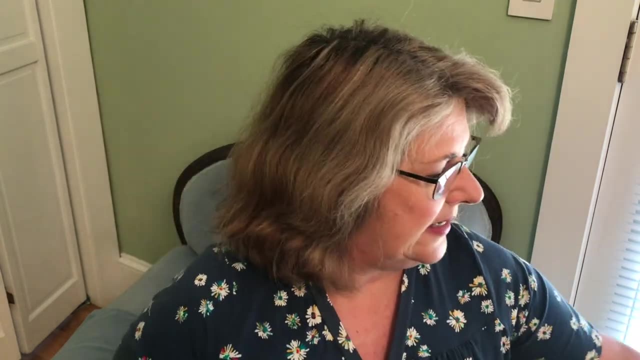 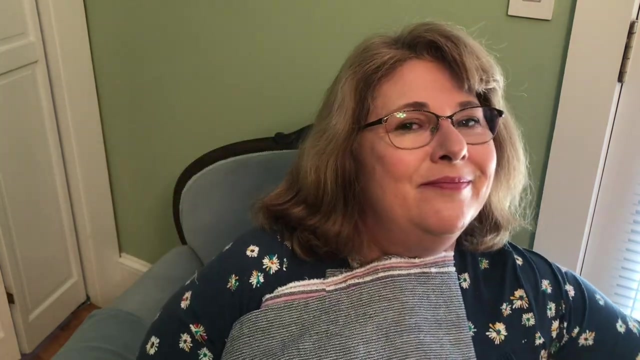 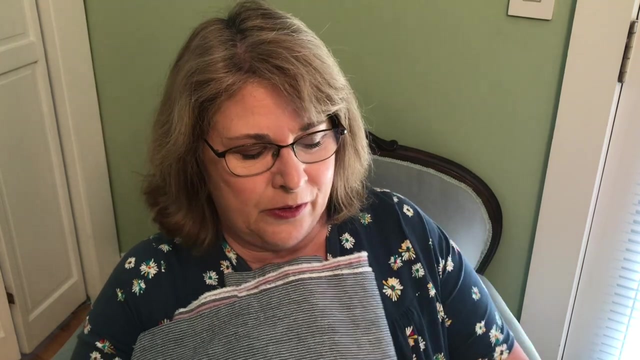 two for baby girl. i think she's gonna need this and i think it would be really cute in a linen. so i have several linens in my stash. i have some pink, bright and cheerful. i've got this pickle color that i think would just be so cute for spring and summer. so my plan: 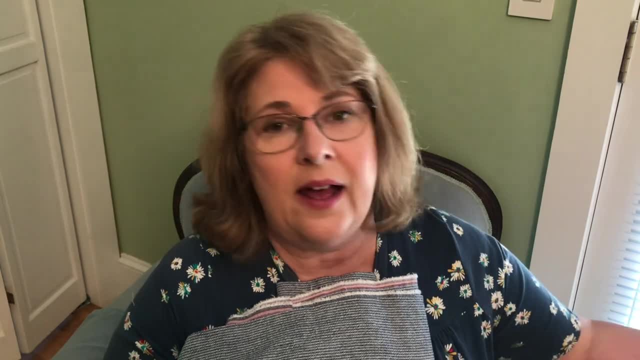 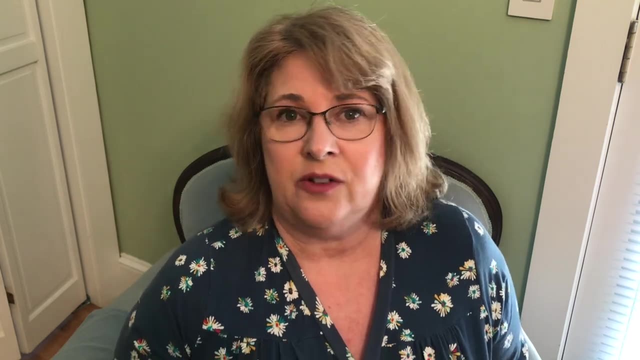 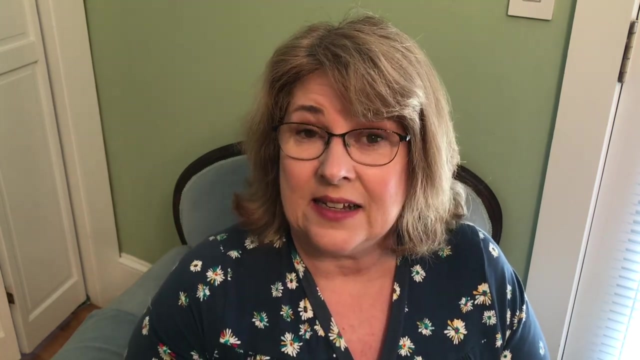 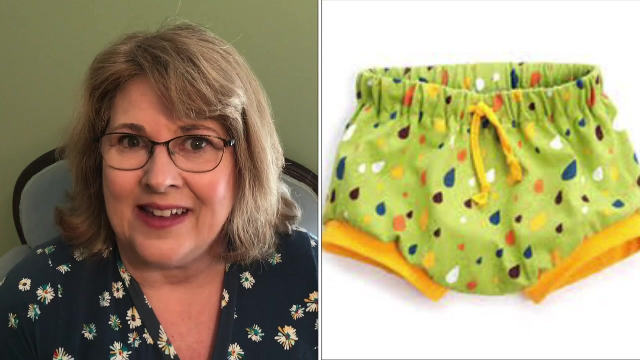 is to just sew the very simple version of the petal wrap. it can be a dress, it can be a tunic and there are pattern pieces to embellish it with really cute pockets, frills, sleeves. but i think i want the very classic, simple version. to pair it with a pair of bummies. brindle and twig has the most adorable bummy pattern i have. 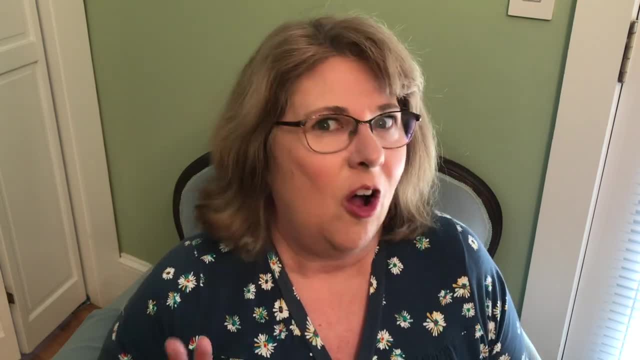 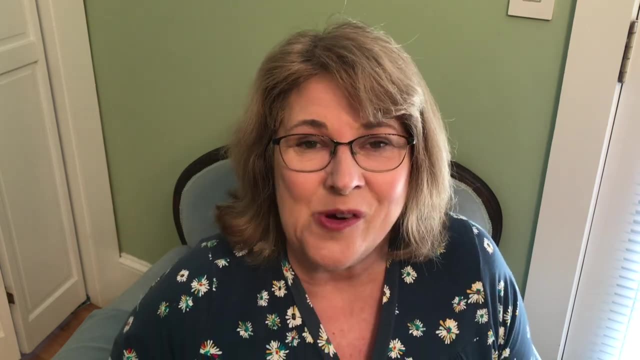 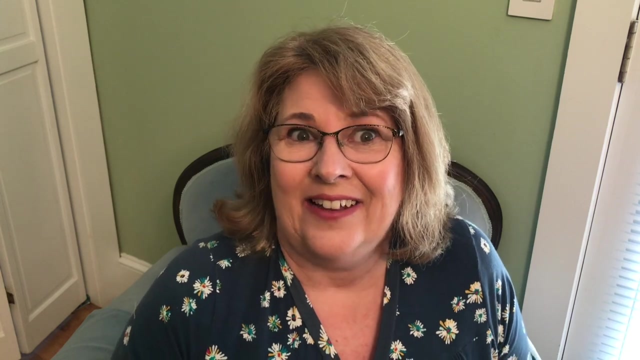 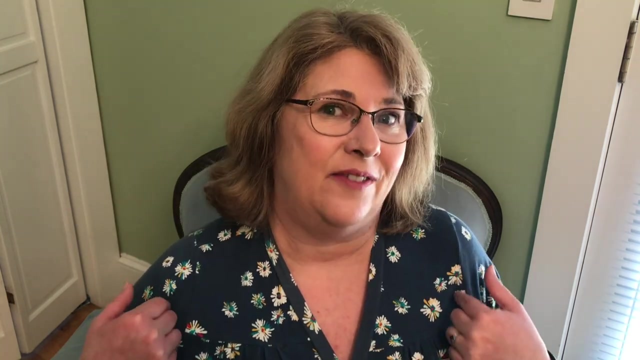 several larger scraps that aren't big enough to make anything for me, and how many pocket linings do i need to save fabric for that? i think i can get some really cute bummies for baby girl and really coordinate well with some of the solid and beautiful patterns that i have, and i have a lot of little ones that i can use to make. 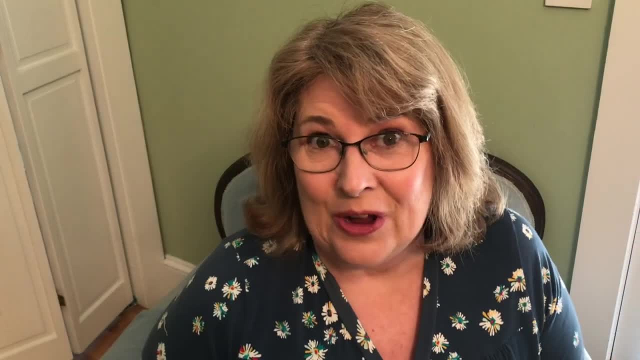 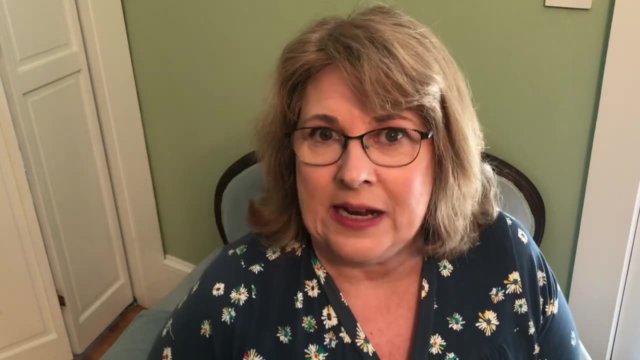 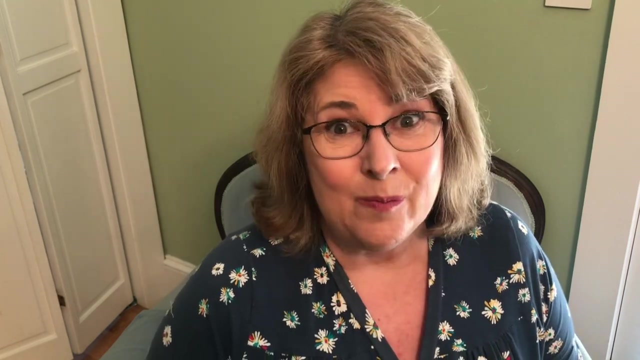 little printed linen that i have in my stash. i do know i have some of this leftover and we could be twinning now we don't want to leave the boys out too. brindle and twig has two hoodie patterns that are free on their website. i have found the brindle and twig patterns to come up a little bit large. 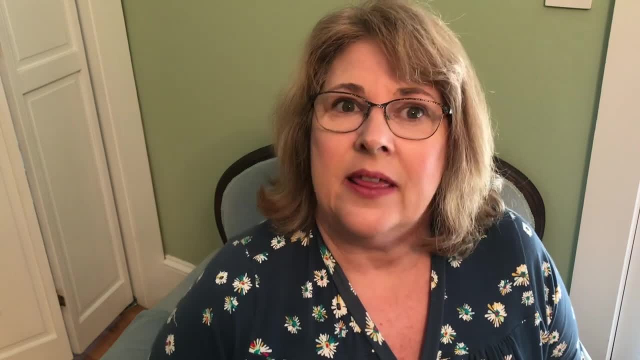 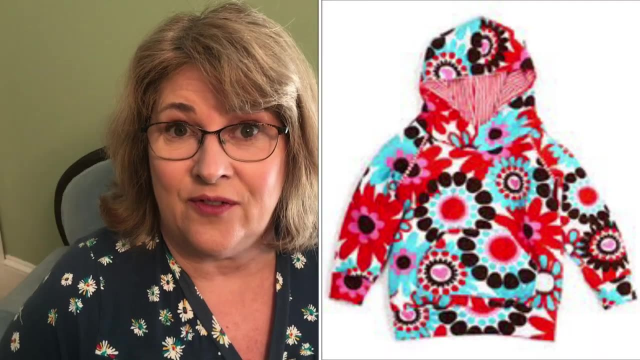 and my littles are not little for their size, they're big for their size. so i'm going to be sewing the scuba hoodie, which is the smaller size range, because I'm going to be sewing a size 5T. but do check out both of the hoodie options. so I picked this out of. 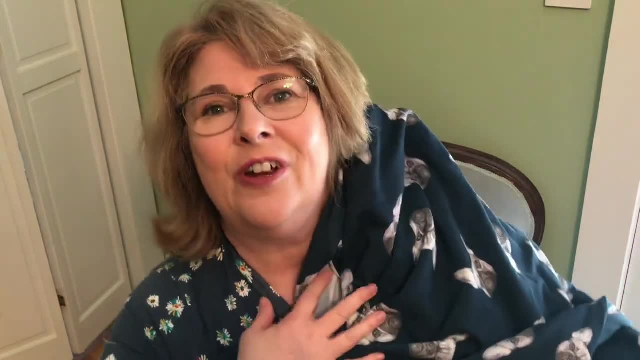 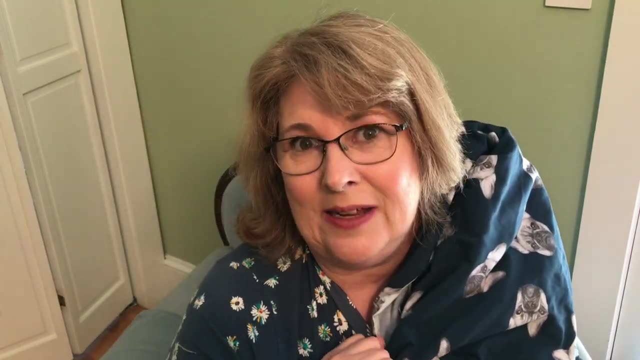 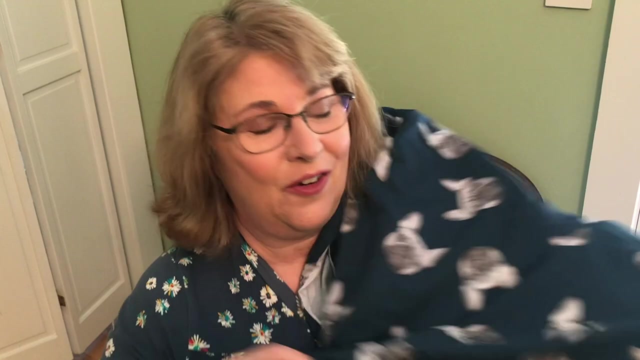 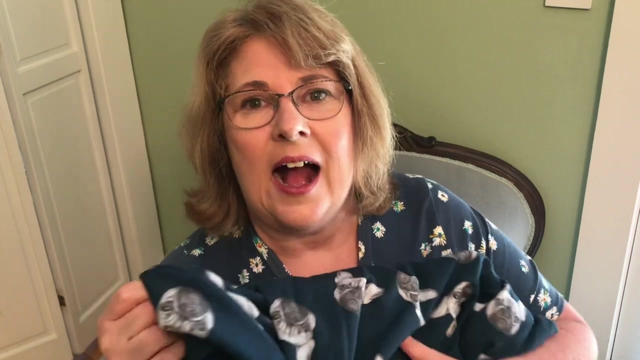 my stash. this is some really cute French terry fabric with French Bulldogs all over it, and I totally blame Adam from Adam Sews for this purchase, or I should say I credit him. this is a very popular fabric and the kids always love to have something with animals on it. I'm going to use some gray cotton jersey that I 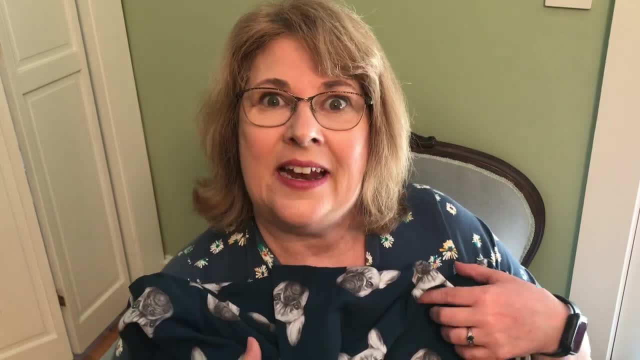 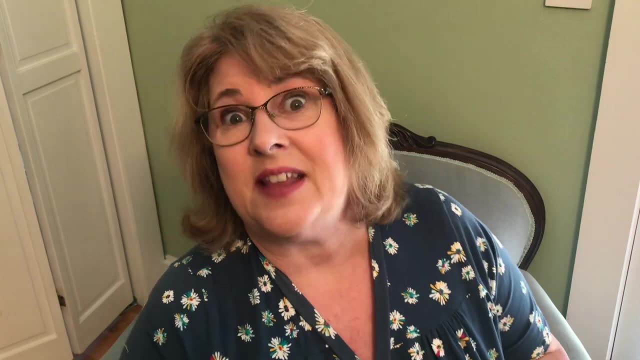 have in my stash to line the hood, and then I have loads of gray ribbing and I think that will coordinate really well with this. so that's the brindle and twig scuba hoodie and, as I said, all of these patterns I'm going to have. 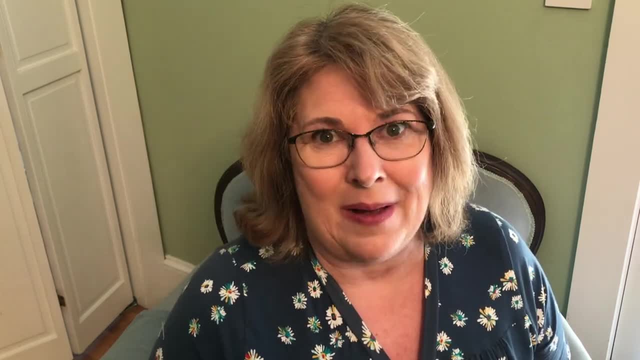 lots and lots of them, and I'm going to have lots and lots and lots of them links below so you can go right to it and get your free patterns. the next pattern I want to talk about is from Polly Woggles, and it's the fathom 5. 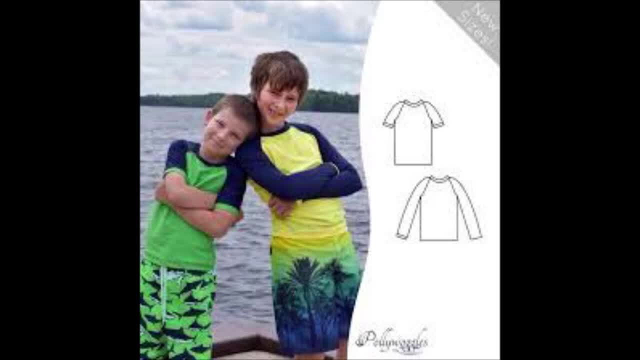 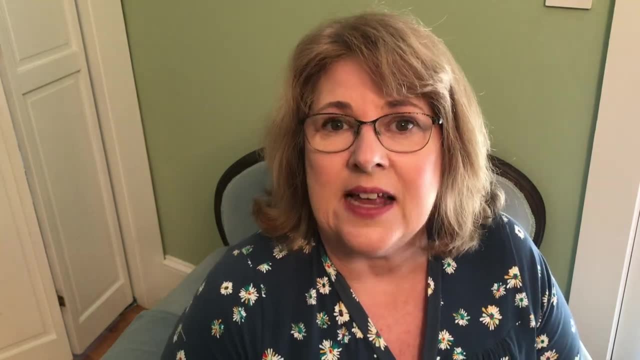 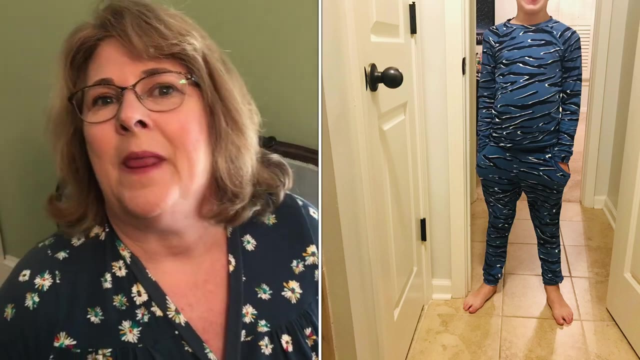 rash guard. last year I sewed this for Sew Frugal and I made it in a size 7 and found it very true to size. I sewed it as a top to a pajama set and I'll insert a photo here if I can find it. I really did like this. 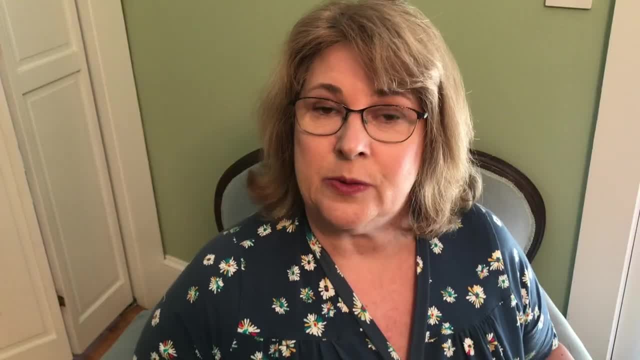 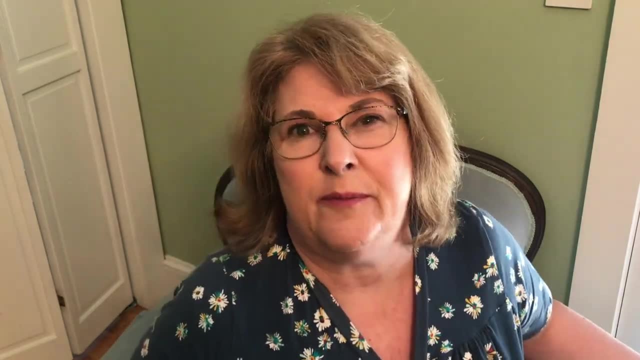 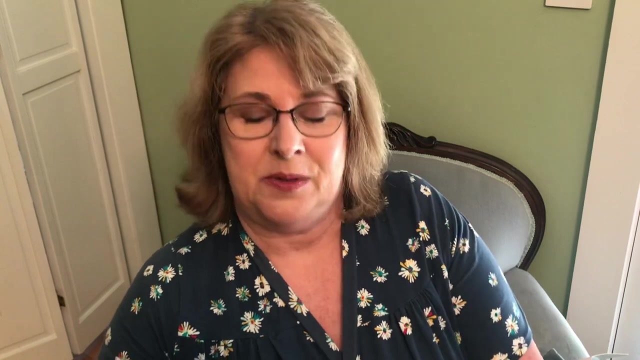 pattern and I thought, now that I have a cover stitch machine, it's time to sew up some rash guards. so I have several swim fabrics that have been in my stash for about three years waiting for me to get that cover stitch machine, and I want to sew up some rash guards and maybe some swimsuits. 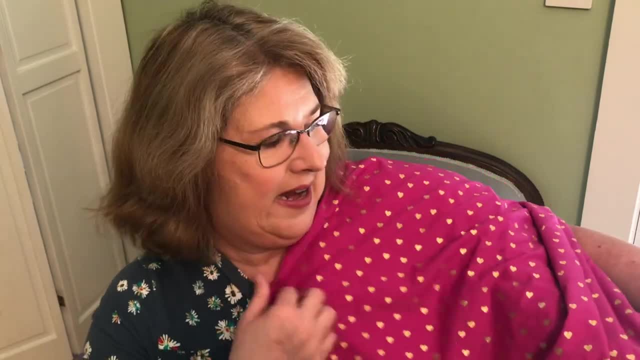 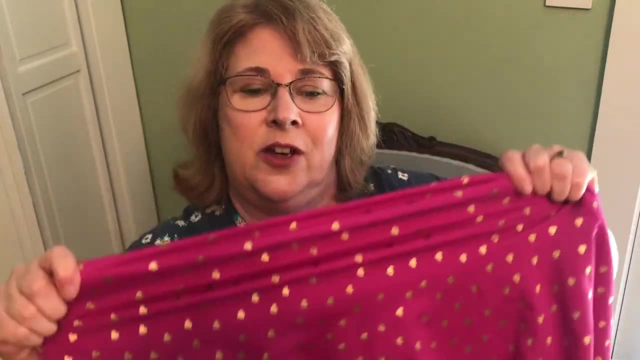 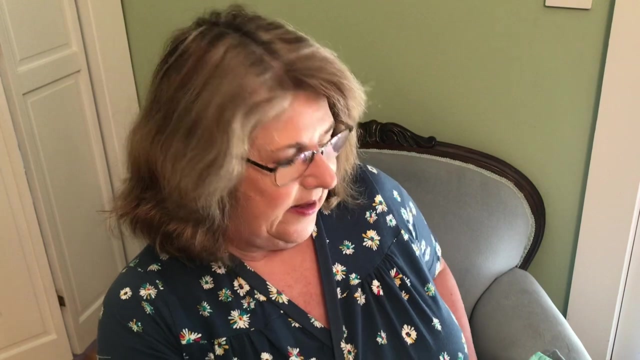 but I think the fathom 5 would look great in this. so I've got this beautiful pink. I got this from Amy fabrics in Pensacola. it's got a lot of stretch and recovery so I think this would make a great rash guard and I think the boys would love one out. 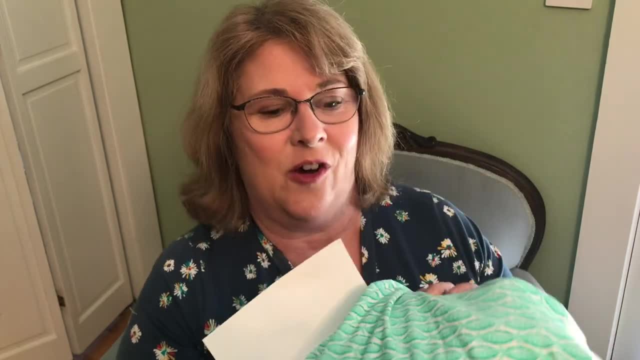 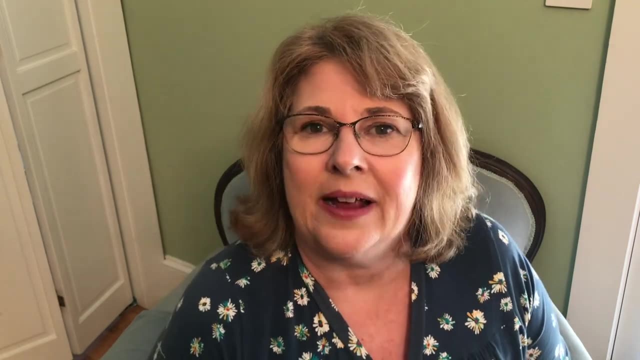 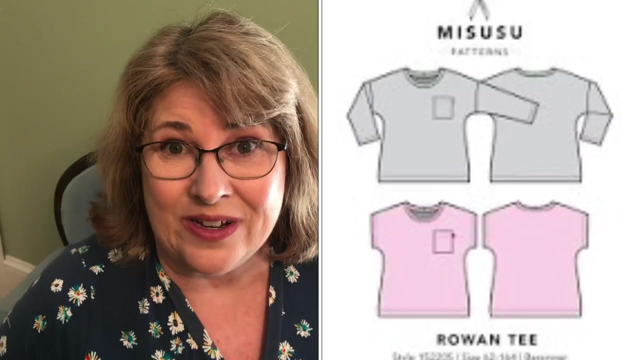 of this? I think they all would. we'll see how far this fabric can go, but it'd be nice to get that sewn up practice a little bit more with my cover stitch machine and I know that that's a great pattern. the final pattern I want to talk about is the Rowan. 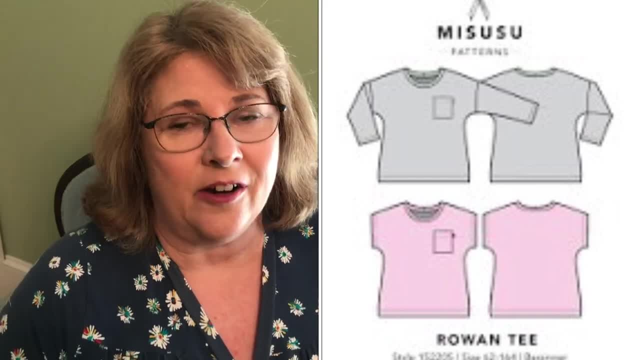 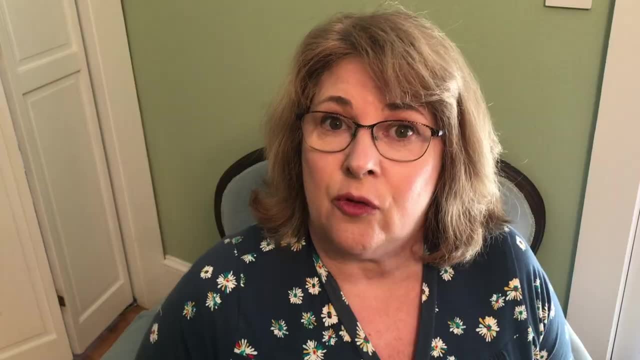 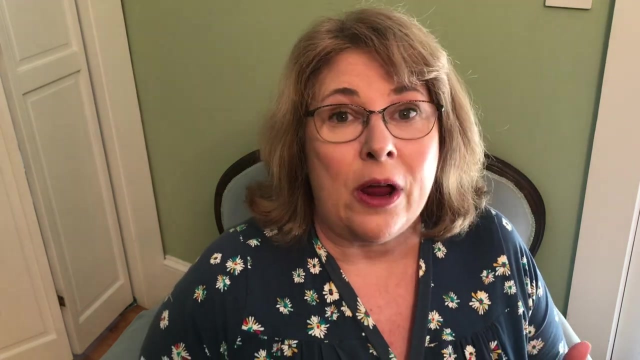 P by Miss Suzu. this is a new to me pattern. I really like the style lines on. it has a drop shoulder and it goes from a size 0 to 14, and I think that this is going to be a must sew for me in March. it'd be a great way to use up all those large scraps that I have.